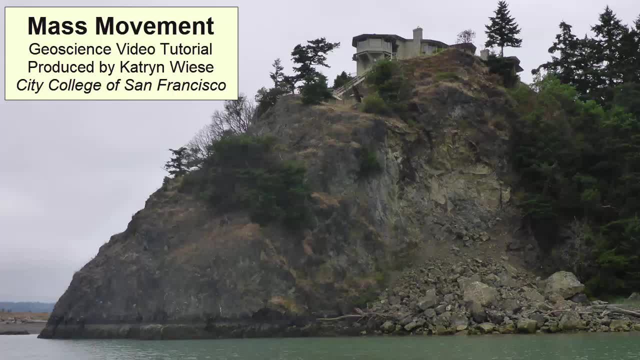 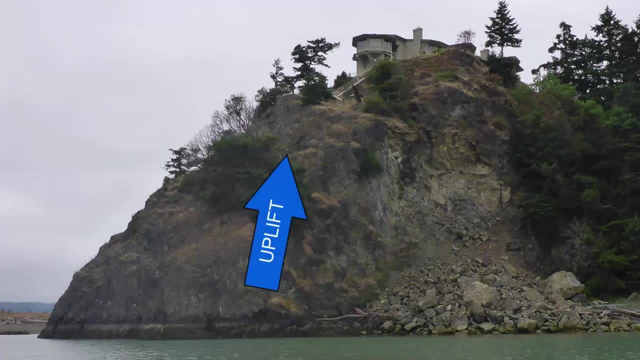 All the landforms on planet Earth are formed through a combination of tectonic forces that push the land up, erosional forces that work to tear it down and rocks of varying character and resistance that impact a location of erosion. To review the term, erosion means the physical removal of rock fragments from one location and transport of them to another location. 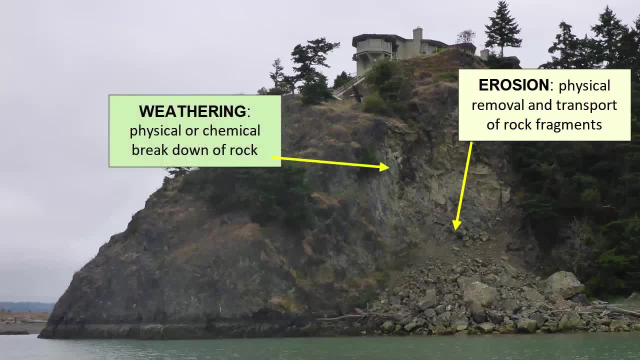 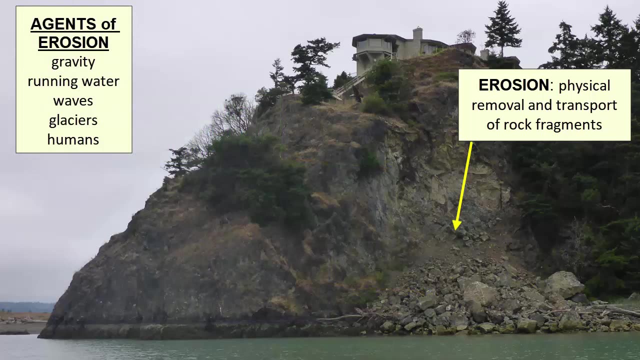 The breaking down of the rock chemically or physically is called weathering. The dropping of rock into a new location is called deposition. In the next few video tutorials, we will focus on various agents of erosion, such as gravity, running water waves, glaciers and humans. 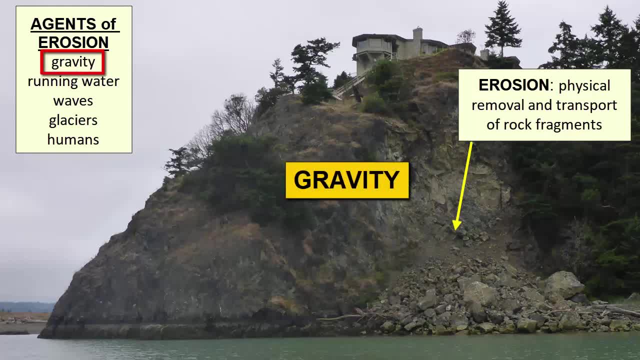 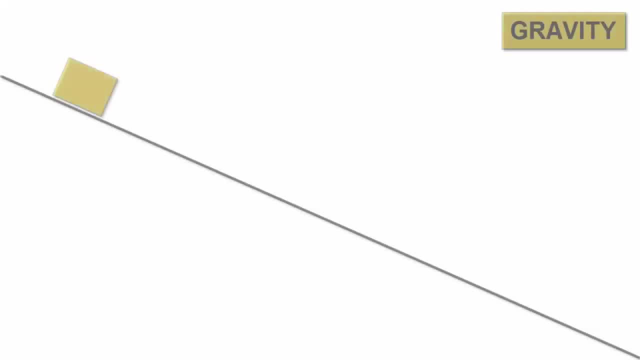 For this video tutorial, we will discuss the erosional agent of gravity. Gravity is a force that pulls material downhill towards the center of the earth. Any object sitting loosely on Earth's surface will feel the pull of gravity and, unimpeded, will simply roll or slide downhill. 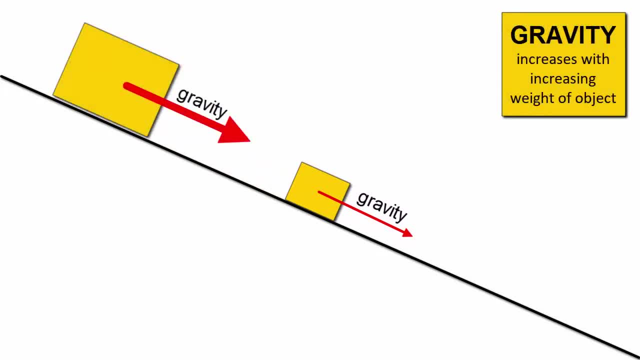 The heavier the object, the greater the force of gravity. Friction is the force that sticks loose material to a surface and needs to be overcome by the force of gravity before objects can move. Friction depends on the materials involved and the angle of the slope. 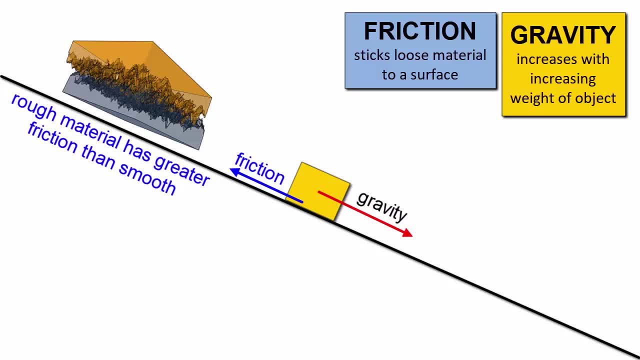 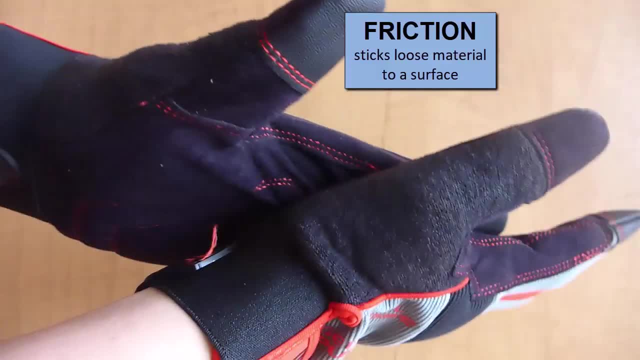 Rough material has more frictional stickiness. Smooth material has more stickiness. Hard material has less stickiness. When my hands are smooth, they slide by each other easily. If I cover them in rough gloves, it gets harder to slide them past each other. 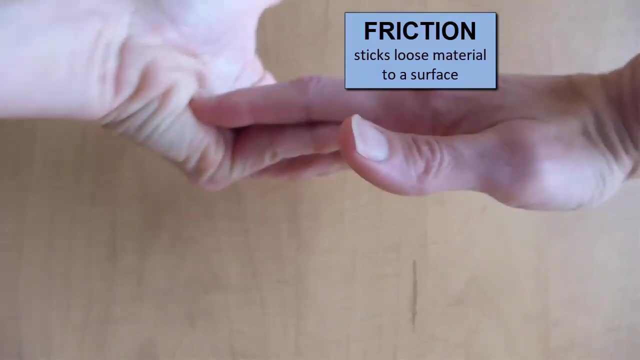 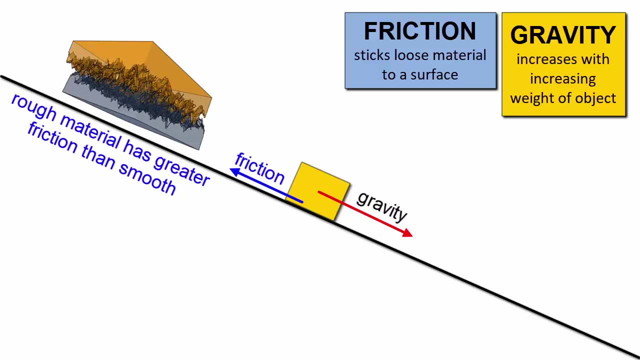 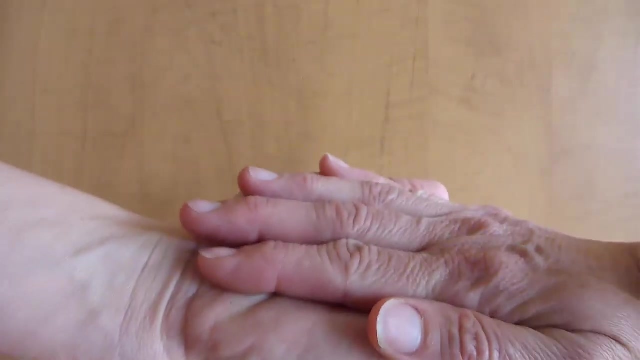 When I bend my hands or let my fingers interfere, it's even harder to slide them. All of these are ways to increase the friction and keep objects from moving downhill. The weight of an object pushing against a surface will also contribute to friction. When I push my hands together tightly, it's harder to slide them. 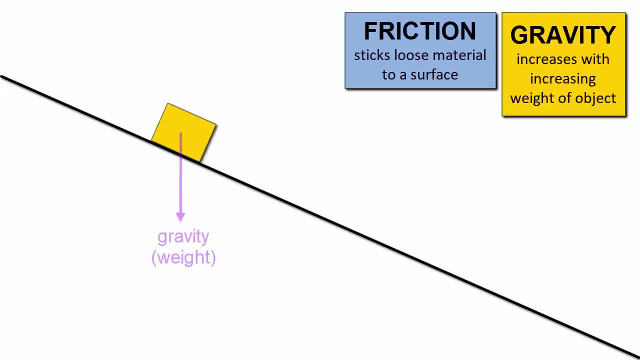 This box, which is sitting on a hillside, is pulled toward the center of the Earth by the force of gravity, which is its weight. If the box is not moving, the component of its weight that moves along the surface of the hill is matched by an equal but opposite force of friction. 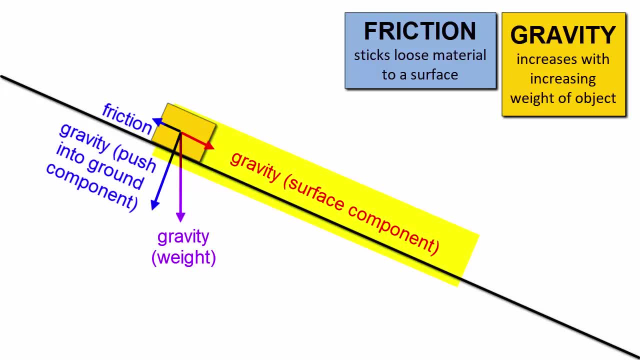 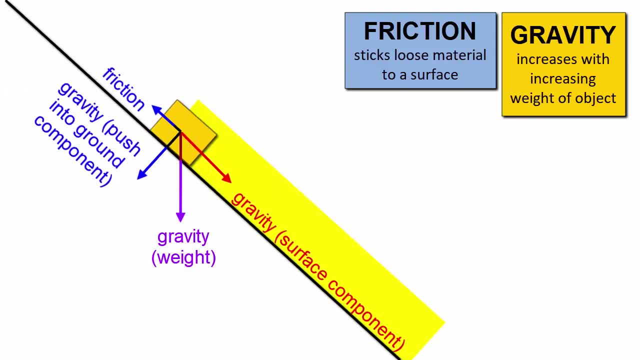 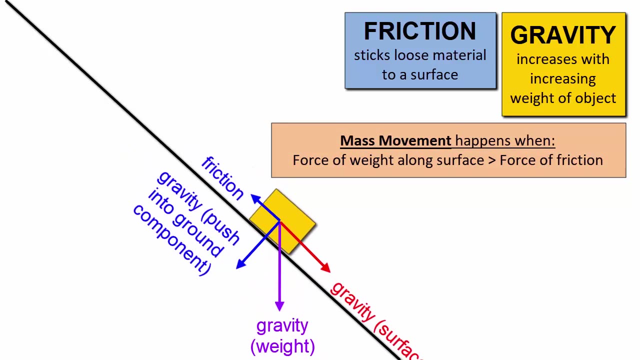 Notice what happens to the force of its weight along the surface. as the hillside steepens, The arrow gets longer, meaning the surface component of the force is getting greater. Once we get the hillside steep enough that the weight component along the surface is greater than the frictional force, the object will move downhill. 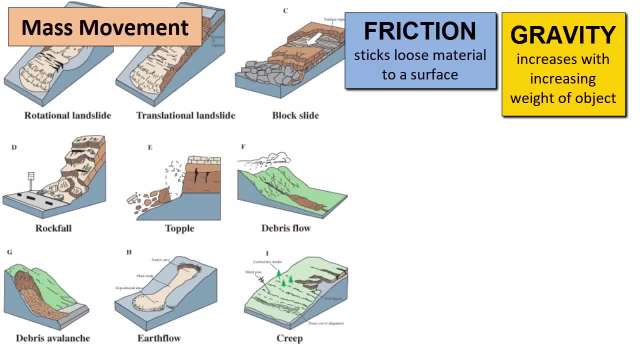 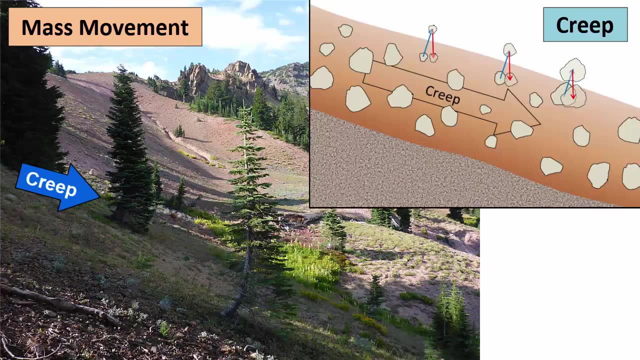 We call downhill movements of weathered rock material on Earth's surface mass movement and we can classify the movement into a variety of types based on the type of material and the way it moves. The slowest type of mass movement is called creep and refers to the topsoil or sediment slowly moving downhill on a day-to-day basis. 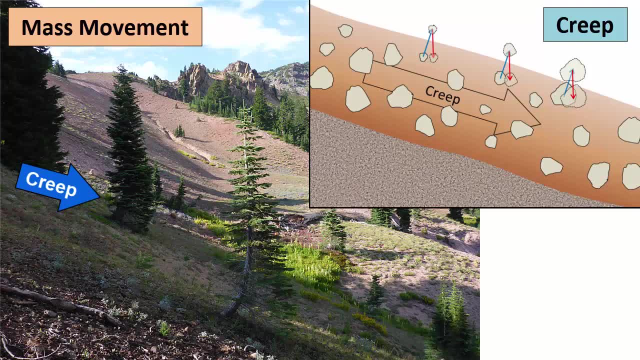 As it alternately expands and contracts through daily heating and cooling cycles. that motion, while happening over distances of less than a millimeter, will overcome small frictional forces and allow a very small downhill movement each daily cycle, Cumulatively over many years, we see the topsoil or sediment layer creeping its way downhill. 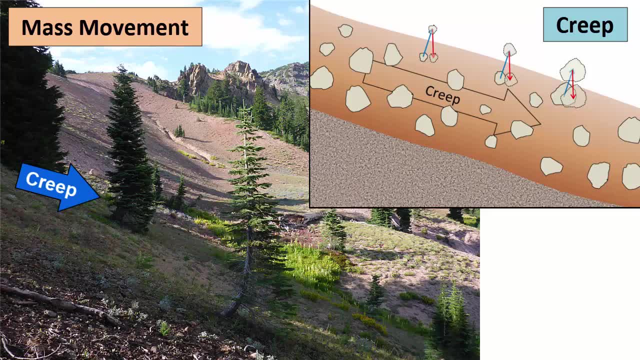 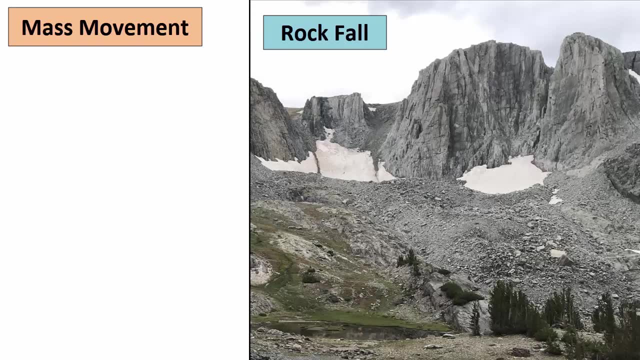 Evidence that creep is occurring is visible when we see trees or fences on a slope bending downhill. The fastest type of mass movement happens during a rock fall, which happens when cracks form on rock cliffs and eventually break off chunks of rock, which fall and collect at the base of the cliff in a pile known as a tailless slope. 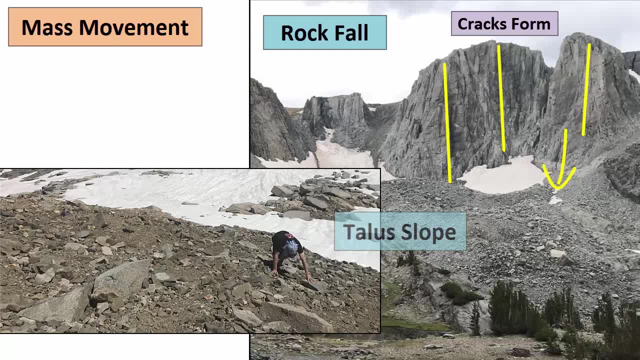 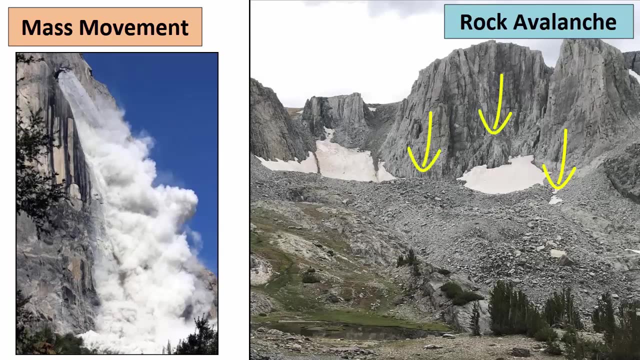 These cracks can form through a number of processes, such as frost, wedging and exfoliation. For more information on the physical weathering processes, watch the video tutorial on weathering, Subtitles by the Amaraorg community. If a large number of rocks fall at the same time, they can trap and ride atop a layer of air. 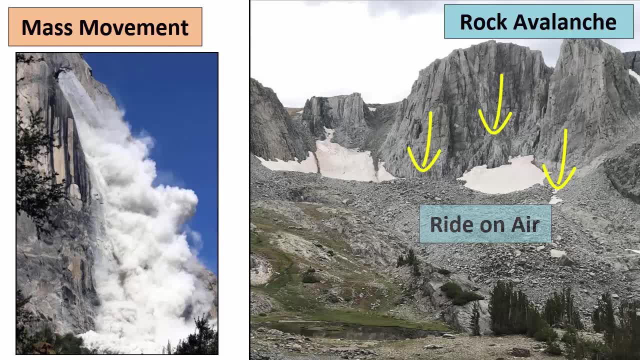 which greatly reduces friction and allows them to move at speeds over 200 miles an hour. We call these movements rock avalanches, and because of their great speed they can travel great distances, even up and over ridges. Rock falls and rock avalanches pose a considerable threat to communities that live in the mountains. 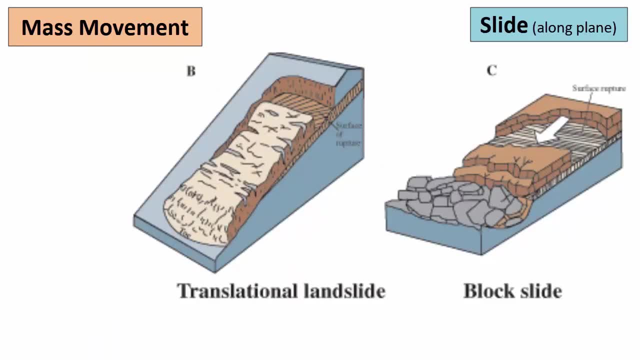 Subtitles by the Amaraorg community. If a rock falls downhill along a planar surface- usually a rock bedding contact fault or foliation plane- it's called a slide. Slides can be triggered when water runs down along the bedding planes, reducing friction between them. 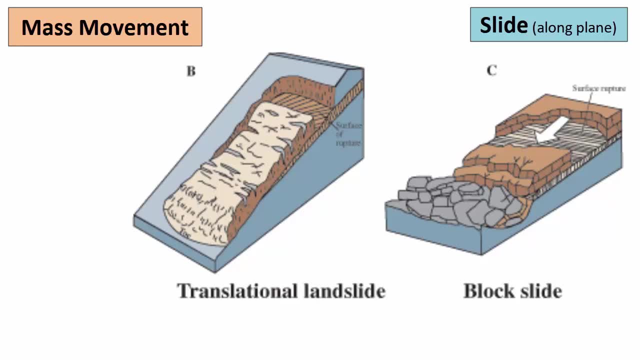 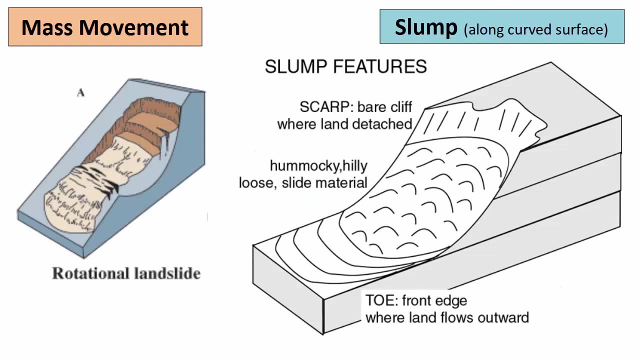 or when the base of the rock bed above the plane is excavated and thus is no longer supported. When material on the hillside moves downhill along a curved surface, it's called a slump. Think about what happens when you slump down in a chair. 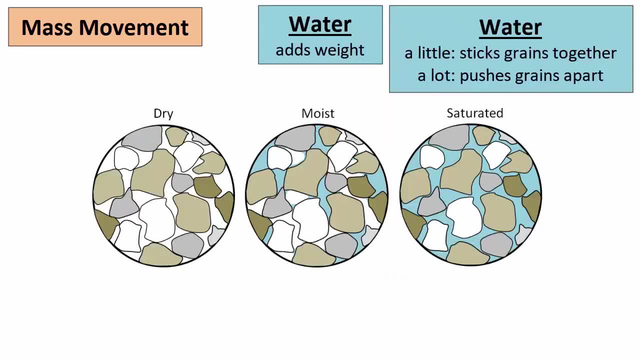 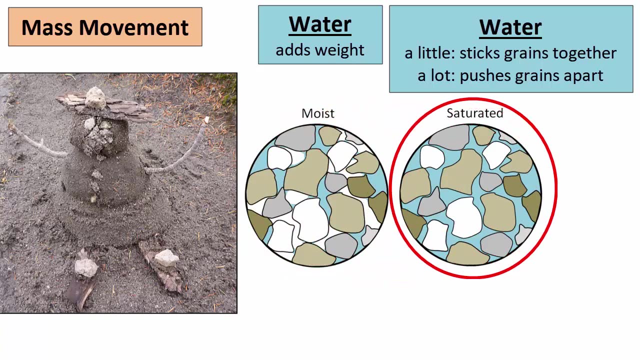 Water can increase the likelihood of all these types of mass movement because it both reduces friction and adds weight. The more weight, the greater the force of gravity. on the hillside, A little bit of water causes small particles to stick together, much like when you build sandcastles on a beach. 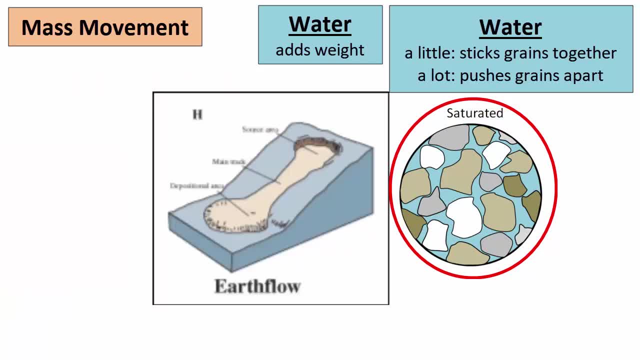 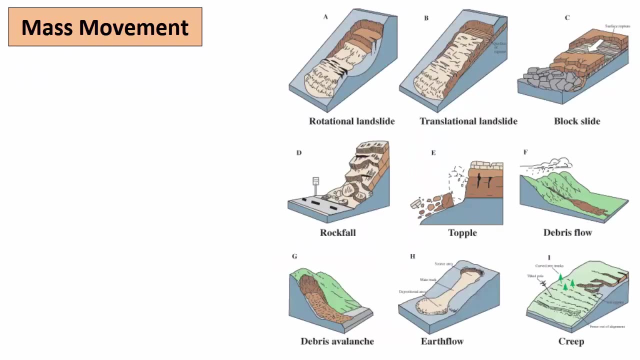 Too much, however, and it pushes them apart. When water content increases enough, it can cause the surface material to liquefy and flow. These types of mass movements where water content is high are called flows. Given enough time, all hillsides will eventually fail and be eroded. 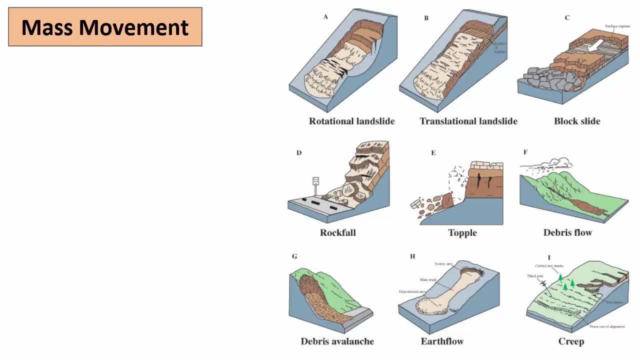 What makes a particular hillside more likely than others to fail? What are some things you can look at, for example, if you're looking to buy property and want to know its stability? First look at the steepness of the hillside. 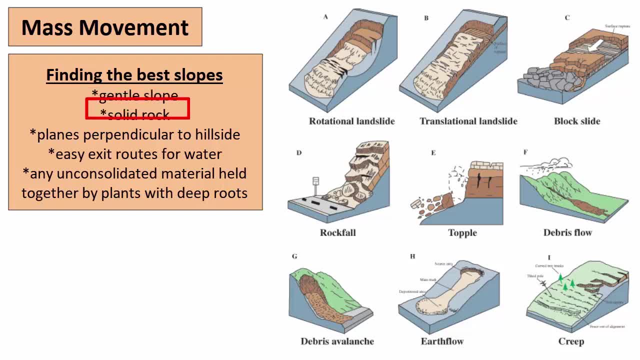 The gentler the slope, the better. Then look at the rocks and material that make up the slope. The more solid the rock, the better. Loose, unconsolidated sediments or soils will be most likely to slump or slide. 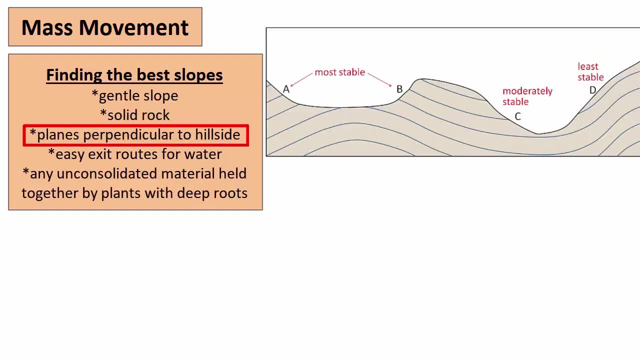 Then look at the geologic structure of the hillside. If there are bedding, foliation or fault planes, are they parallel to the hillside? If so, they are more likely to fail than those that are perpendicular to the hillside. 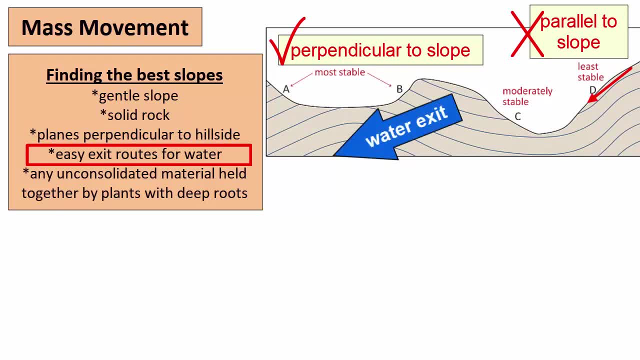 Is there a way for water that penetrates the hillside to easily flow out? Does it sit atop any ponds? Are there any springs? Water adds weight, so the more easily water can hit the surface and safely run off, the better. Finally, look at the vegetation. 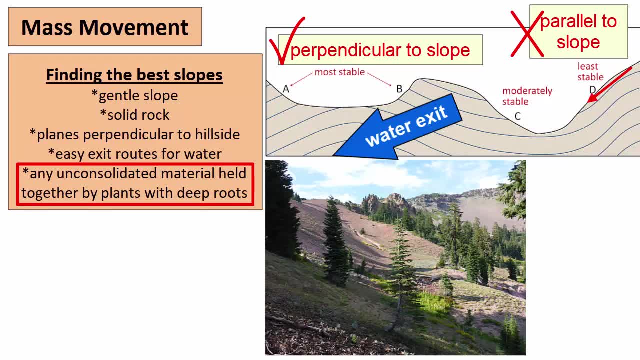 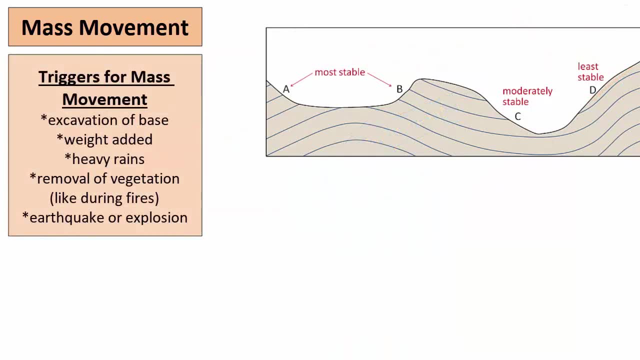 Plants with roots can help keep soils more compacted and connected, especially if the roots are deep. What are some triggers that could start mass movement on a susceptible hillside? When the base of a rock bed is excavated, it loses its support. 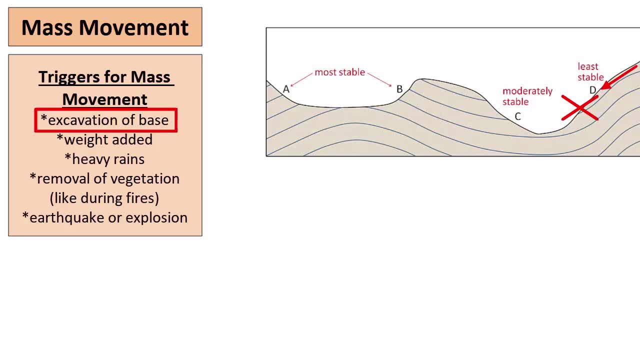 Excavation can happen during building of highways or roads or houses, Or when rivers flood. Weight added to the top of the hillside will increase the force pushing downhill. Weight is added when houses are built on the top of a hill or when excavated sediment is piled up on top of the hillside. 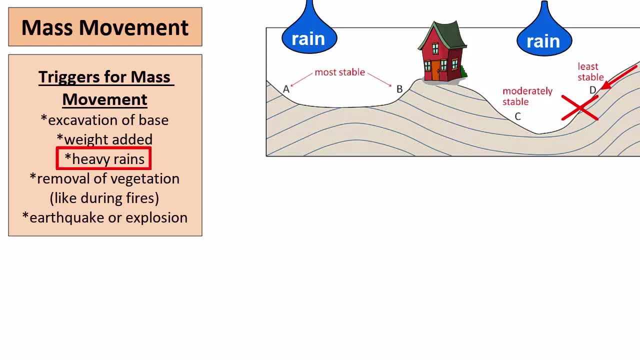 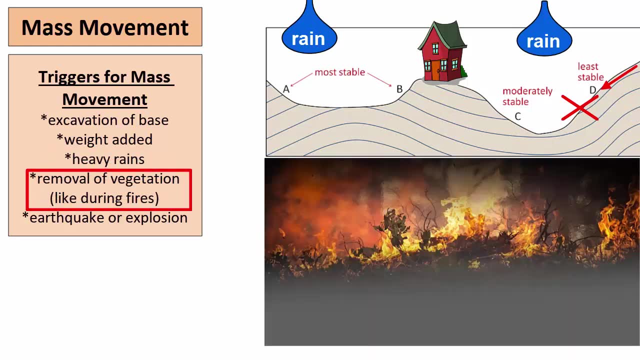